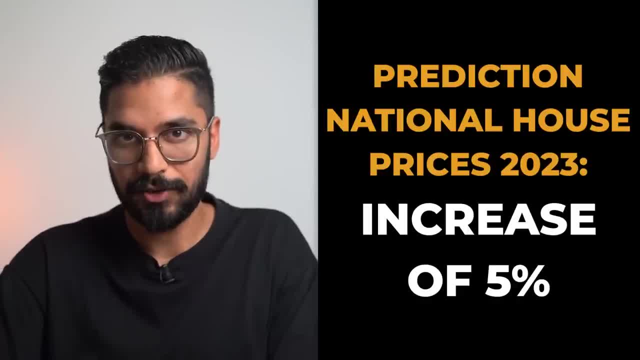 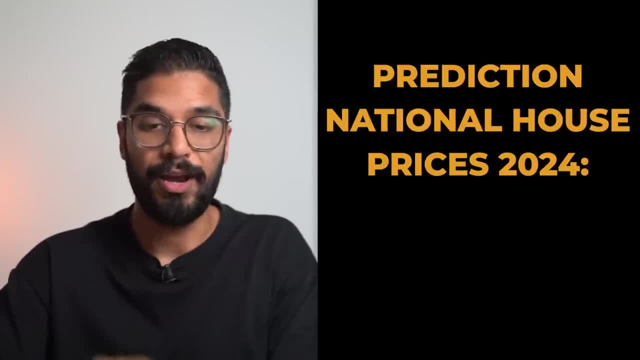 largely going to be determined by how fast the interest rates start decreasing. It could be a lot more than that if we decrease by more than 50 basis points in 2023.. In 2024, I think we're going to go and almost 2x that and we'll grow by 9%- And I know these numbers are sounding pretty. 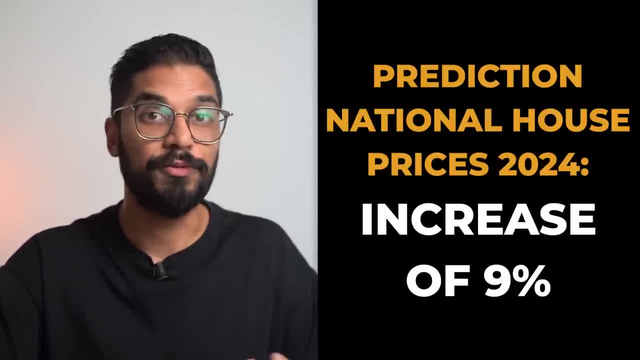 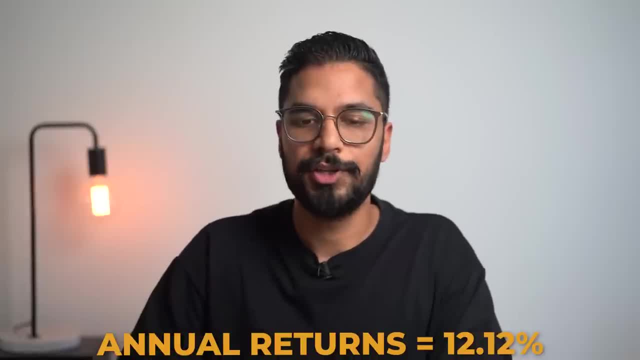 crazy On a property that's worth $500,000, that's an extra $45,000 next year. Now, in terms of the buyers agency that I run at, Search Property, our average result in terms of annualized returns was 12.12%- Absolutely mind-blowing, And I'm so happy and grateful for. 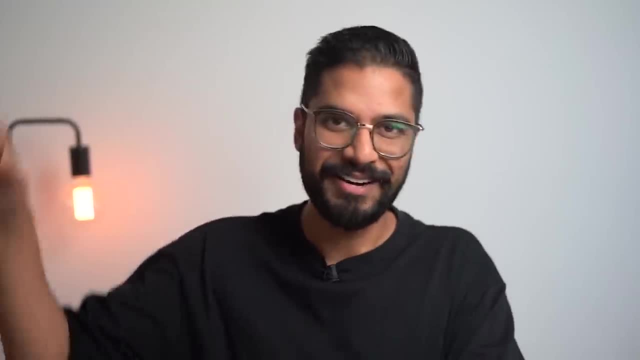 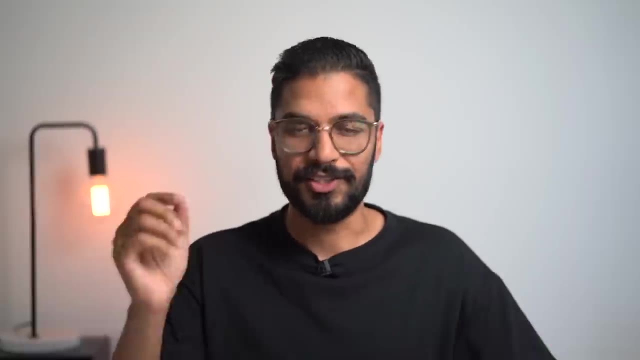 the team, Our research actually works, even in a market that's taking off and in a market that's going down, because we know in 2022, the markets did decline by 7.1%, but we outperformed it and we actually grew. So the clients are very happy, naturally, why they want to sign up again. What's? 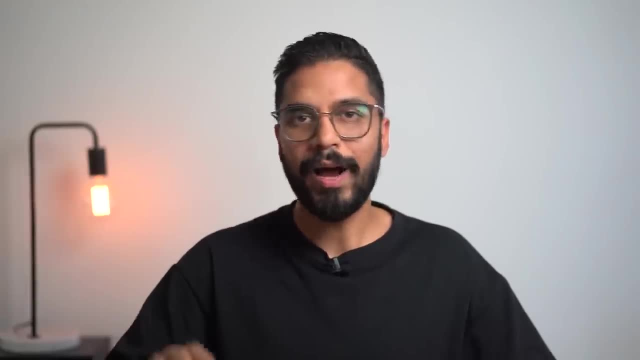 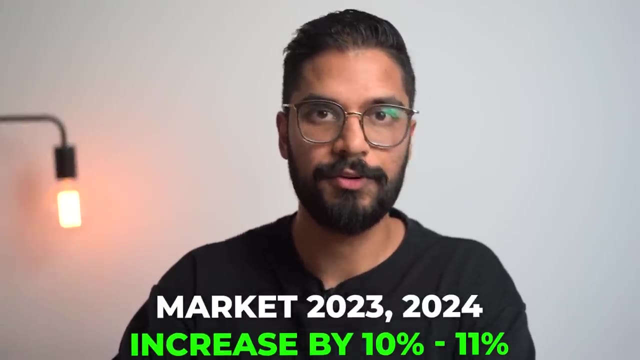 up In 2023 and 2024, I believe, yet again we will outperform, whatever the national average is. So I am expecting a minimum of 10% to 11% in 2023 and in 2024.. Now, that's from a capital growth. 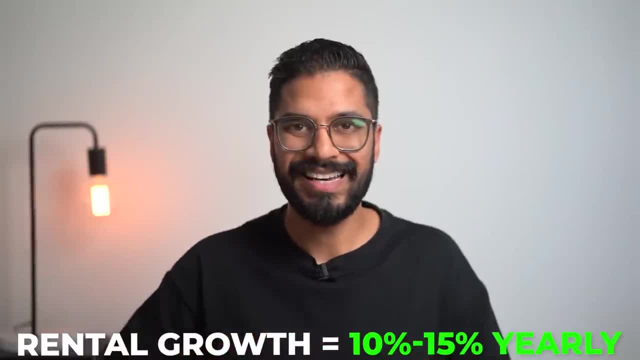 perspective Where I think rents will be going is about 10% to 15% year on year. So I don't just think it's going to go up by 10% in 2023 and then level out. I think it's going to increase by 10%. to 15% in 2023. And then we're going to see another increase of 10% to 15% in 2024.. So you could see rents anywhere between 20% and 30% higher than where they are today. I know it sounds. 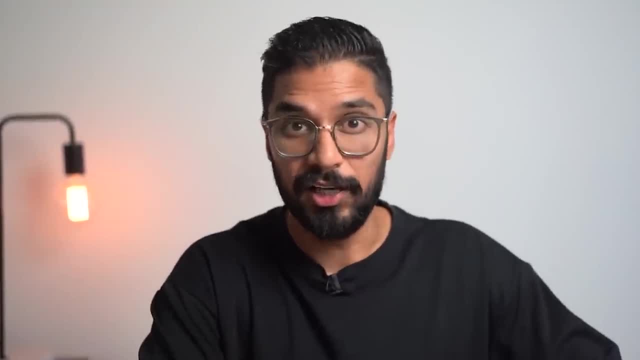 crazy, and it often does before things take off. Trust me, I'm not going to lie to you. I'm not going to lie to you. Trust me, I sounded like a loony in April 2020.. Go check out this video. 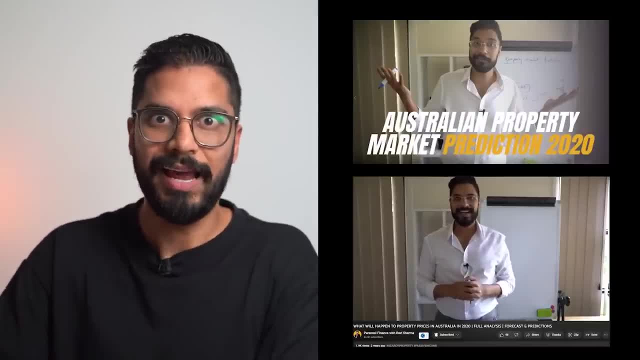 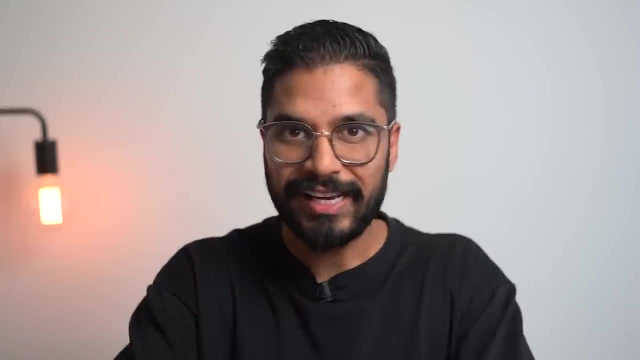 where I was basically predicting what was going to happen with the property boom and it did play out. And trust me, at that time it sounded crazy even when I was writing it, but I'm like. the logic makes sense: The market doesn't care about my feelings, just like it does about this. 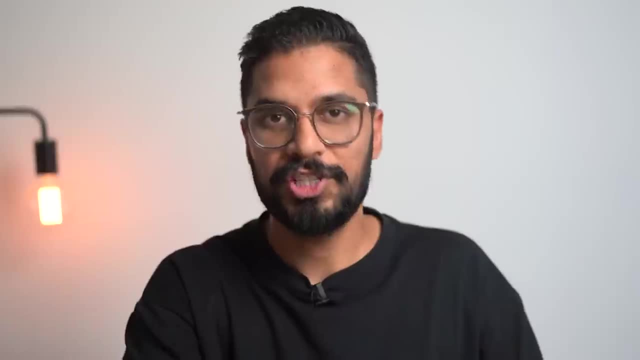 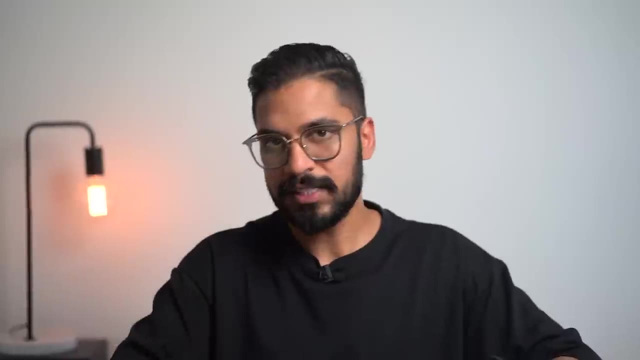 If I'm making these predictions is based on a lot of stats, a lot of graphs, and I'm going to share with you a couple of those because I don't want you to get bored. after like a 50 minute video, You're going to be like dude, I hate this guy, But anyways, let's continue Now, when it comes. 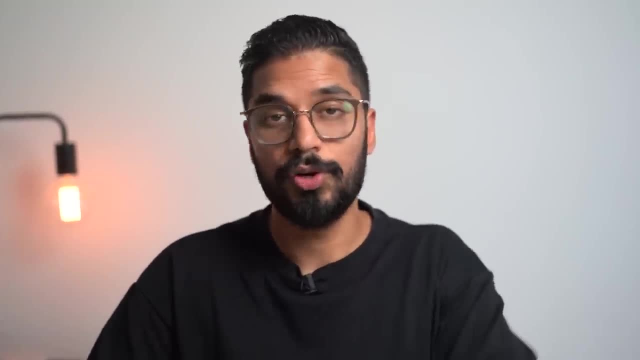 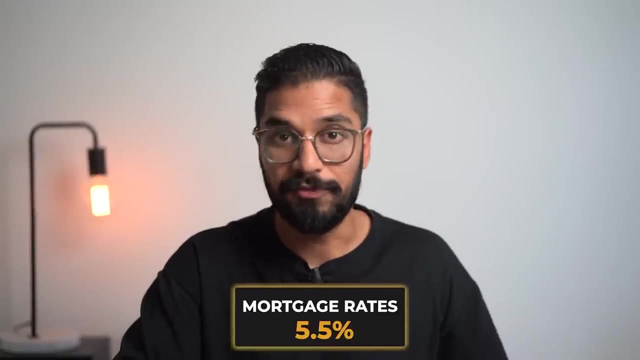 to interest rates. this will not only be driven by what happens in Australia, but also what happens, So take this with a grain of salt, but I believe these are going to be fairly accurate. Mortgage rates at the moment are at about 5.5% and I think this is basically the peak. I think, by the end of 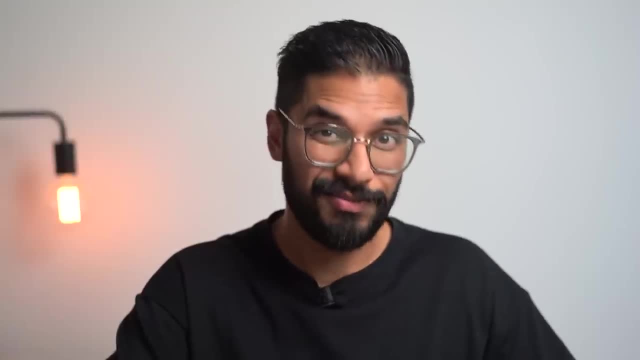 2024, so almost about 18 to 24 months from this video being shot, we will see rates closer to 3 to 3.5%. Now that's the mortgage rate. If you look at the cash rate, we're in the low threes at the. 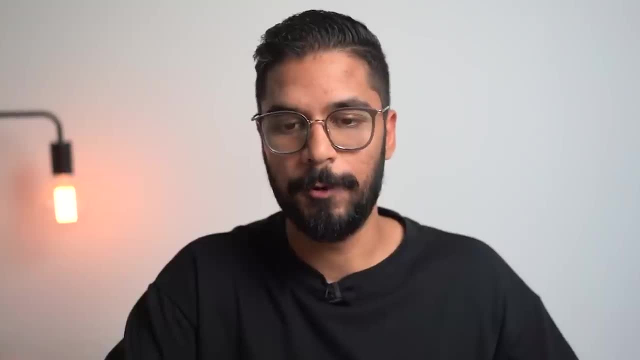 moment. I think we will fall back into the low twos, if not enter the ones as well. Now let's jump into three graphs that I want to show you. that's going to showcase exactly what I'm looking at and forms part of the research that's helped me determine. 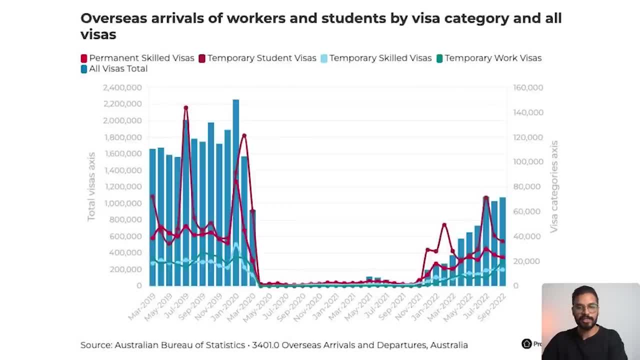 how far property prices will actually go up. The first one here you'll see is overseas arrivals of workers and students by visa category and all visas. What you'll see is that, basically, between May 2020 all the way through to November 2021, there was little to no people coming into this. 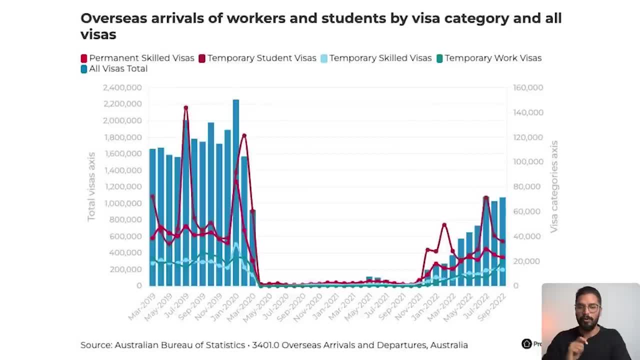 country, And why? Because we had the pandemic, we had the borders shut off, right. But what we're starting to see is the increase- and it's a rapid increase- in the overseas migration. So take a step back and understand that we're not even at levels that we saw prior to the pandemic in 2019.. So 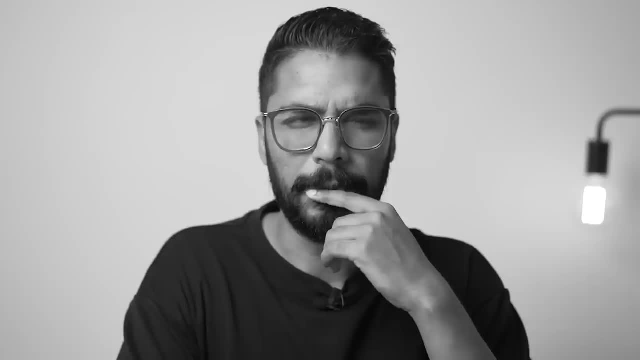 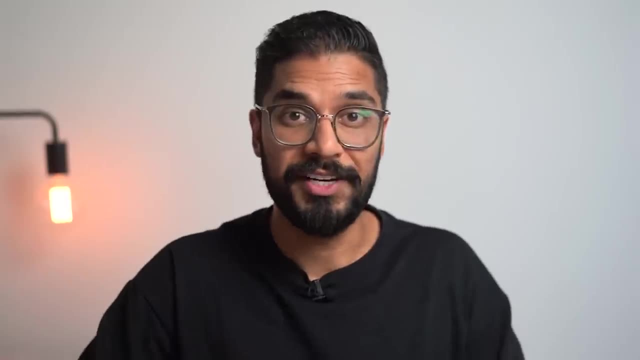 we're going to eclipse it by a lot. I know you could be sitting there and be like, but hold up. if immigrants are coming into this country and we already have a rental crisis, where is everyone going to live? It's a fairly good observation because it's the truth. Now there are still. 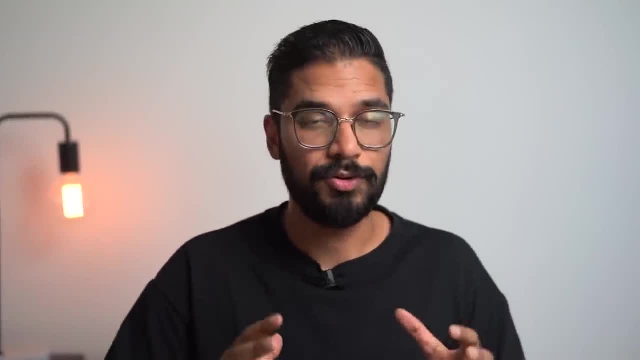 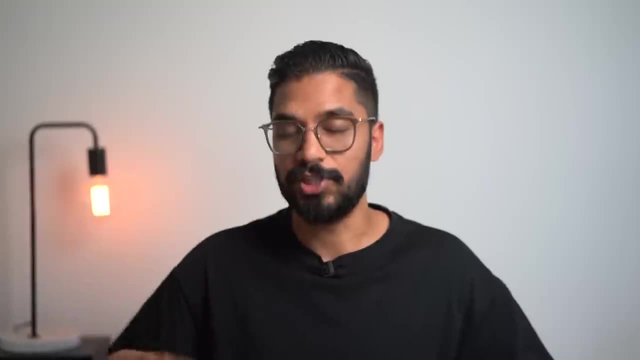 properties available in a lot of different pockets, but you'll start seeing that rental crisis increase exponentially in certain areas And the government at this point is not stepping in with little to no help when it comes to rental subsidies, which I think they should bring. But 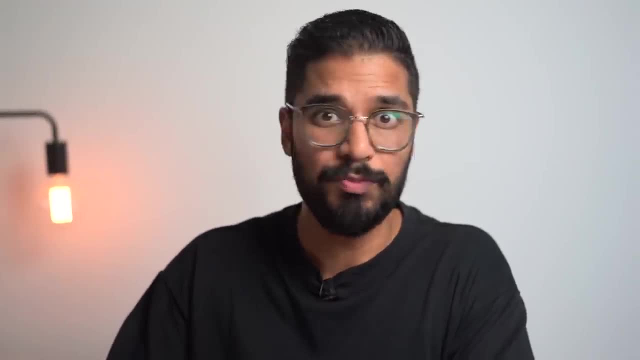 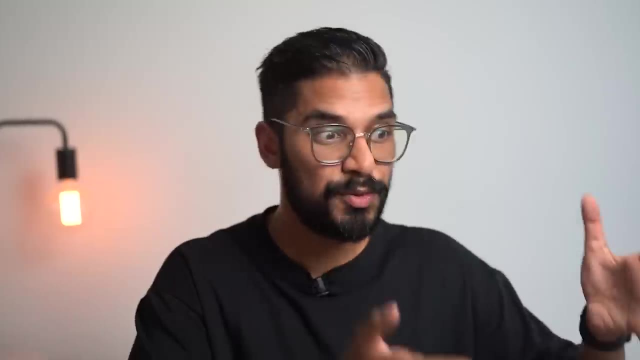 more importantly, their approach is like: if you don't want to live there, just move to another suburb, which I definitely don't agree with. but that's the reality. And again, the market doesn't care about my thoughts. It definitely doesn't care about your thoughts, So you may as well know the 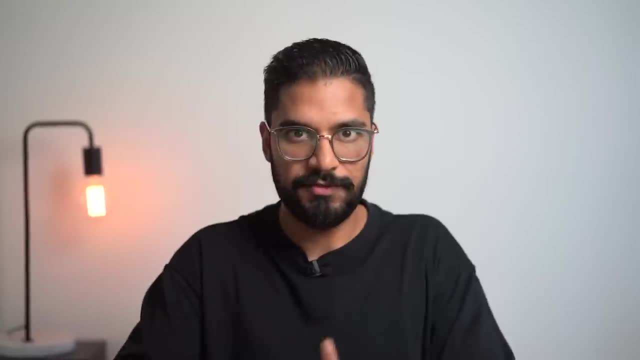 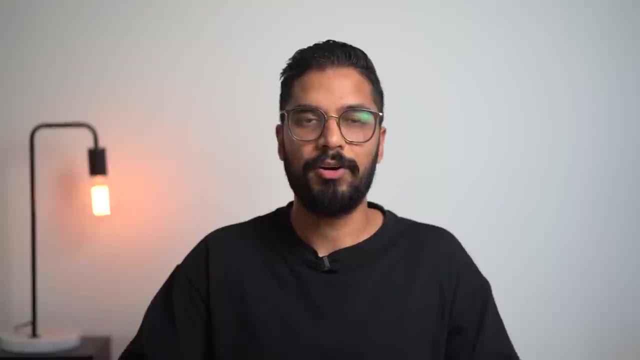 rules of the game: adapt or die, unfortunately. So if we know this information, we can then go ahead and say we want to target areas where we can see significant amount of growth because there's no supply there Now, contrary to people coming out and saying: well, this guy's an evil. 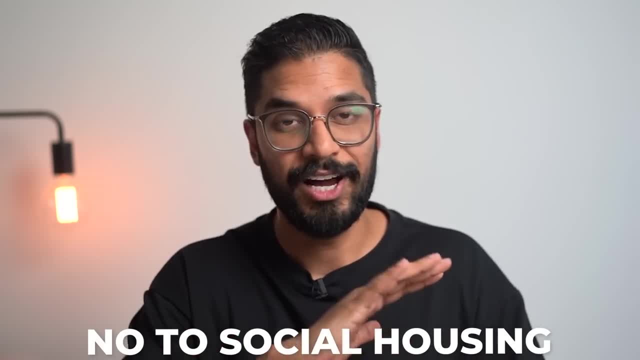 investor- and this is so bad One- I don't go into social housing. I think that's ethically so wrong. I wouldn't do that When I'm going in and purchasing in a location a lot of the properties that we're. 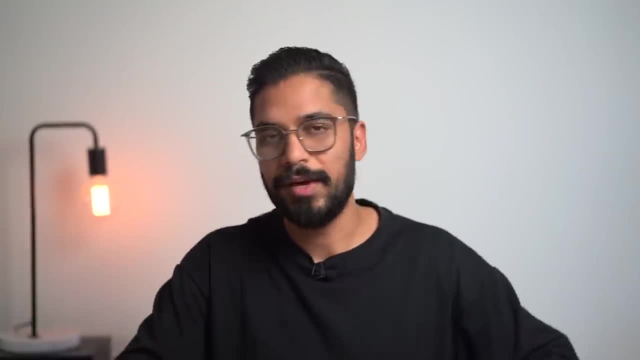 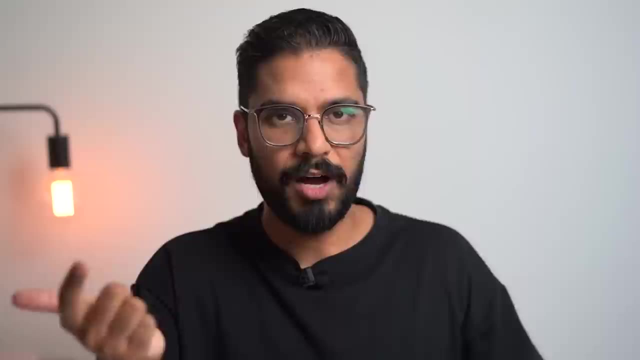 are from owner occupies, So they might be going and downsizing, They may be moving to another area, They may be moving overseas. So when you go ahead and target owner occupy properties, one, they're better kept, but also two, I'm going out there and providing more supply to the rental. 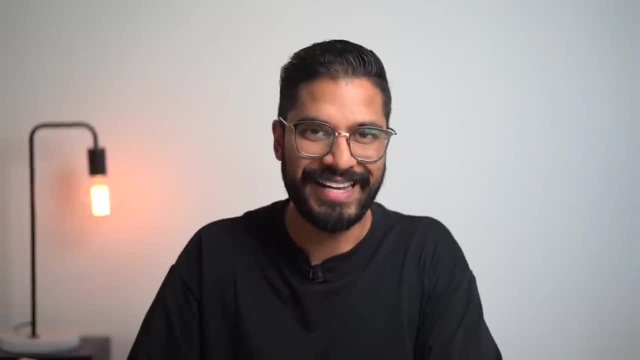 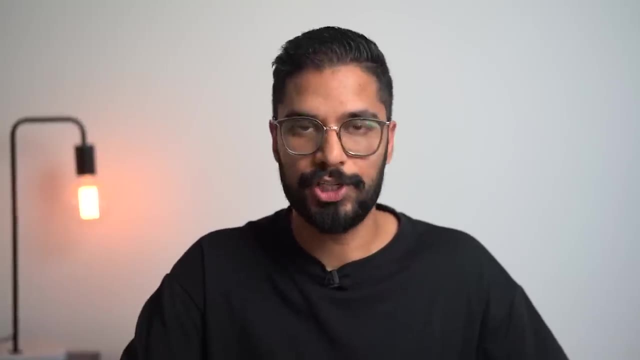 issue. So again, you're not going to be able to please everyone. I'm definitely going to get negative comments anyway. but the whole idea is, if you're going to look at this strategically for your own financial freedom, for your own financial wealth, then this is a very important chart to 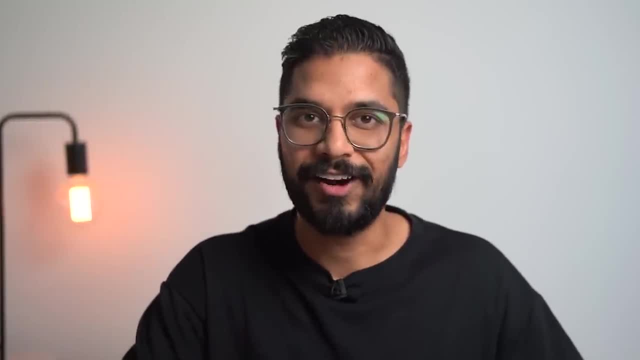 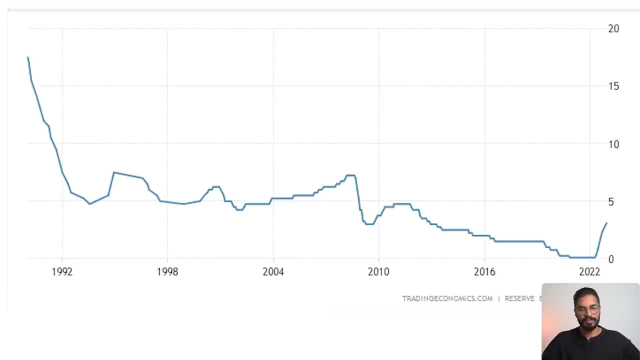 know because of how many people are coming into the country and you've got to then figure out where exactly are they going. The next graph I've got for you is the Australian cash rate from 1992 over the last 30 to 35 years. 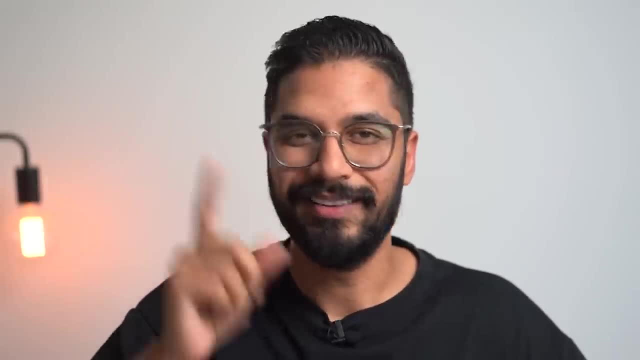 Now, I was born in 1992.. So I know that was 30 years straight off the top of my head. I'm turning 31 this year, But what we're seeing here is only one thing, which is the graph continues to go. 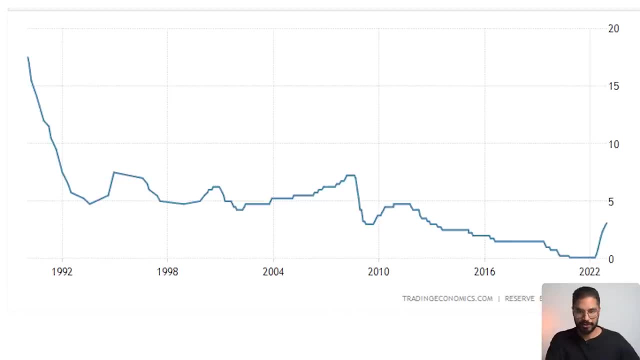 lower. Yes, we're going to see periods of spikes and we've seen that throughout the last 30 to 35 years And more recently, we've had the increase right now, In 2022,. we've had increases in rates so quickly like we've never seen before. But what's important here and what I want you to take? 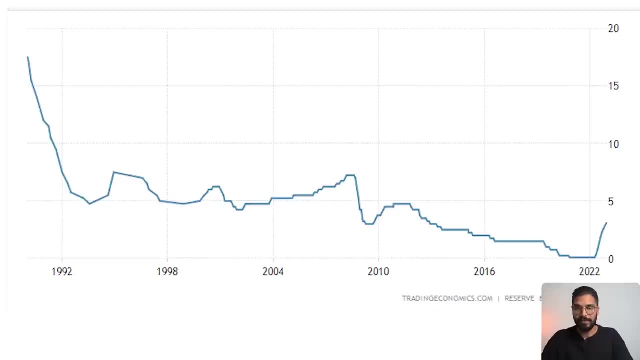 away from this is that when we get close to the peak- and I believe we're already there, and if we are, then we don't spend longer than six to 12 months at that peak- At that point we're going to start cutting, And what you'll see at every single point in the last 35 years, every time. 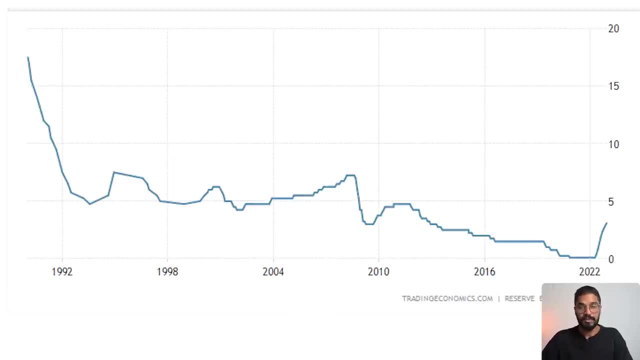 we've increased rates, we drop faster than what we've increased. Now this time might be different and I think it might resemble something closer to what happened in 1995 to about 1997.. And what we could see is that I don't expect rates to drop for nine months consecutively and at the pace that 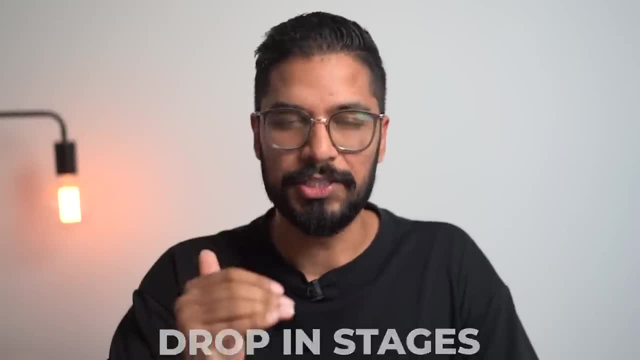 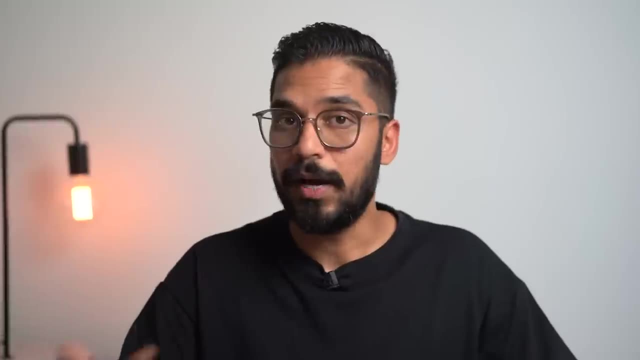 they did. Instead, what I'm thinking is going to happen is they'll drop in stages And what we might see is they drop initially by 50 basis points, Then over the next six months, we see them drop by another 100 basis points And eventually, I believe we're going to have 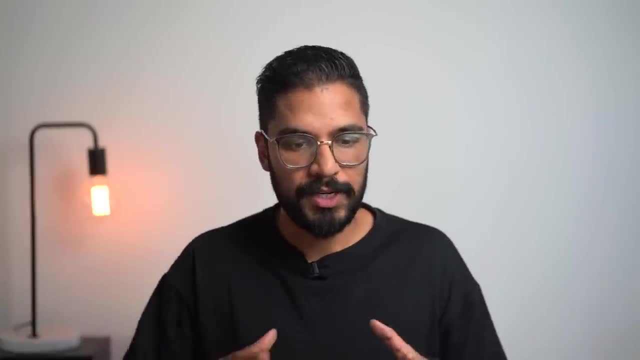 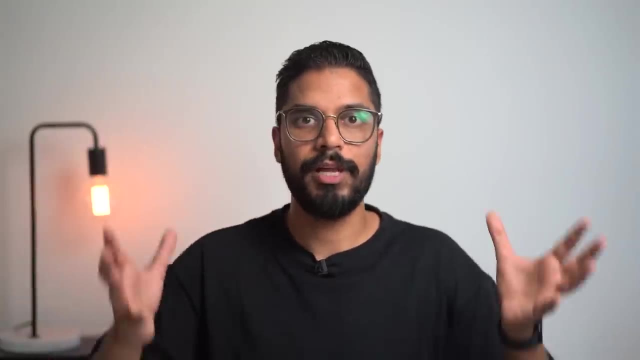 interest rates go back close to zero again, And the reason for that is because the entire system, the entire monetary policy, is based on this debt-based system. It's the devaluation of our currency. It makes everyone feel like they're wealthier. They actually aim for two to three. 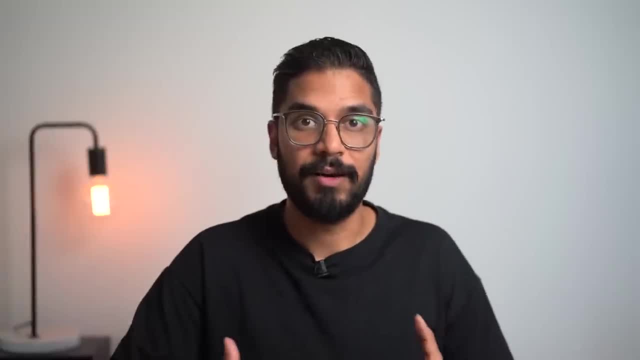 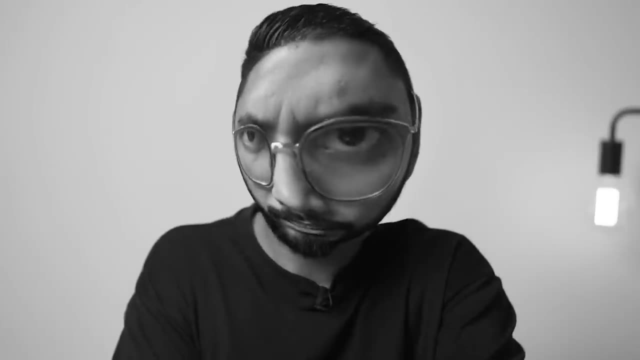 percent of inflation every single year. So, although inflation is something that you might have come in your grocery bill, it's what they aim for every single year. So there you go. Well, yes, you work here in Australia. This is the tax you pay, which is like 20, 30 percent in some cases. 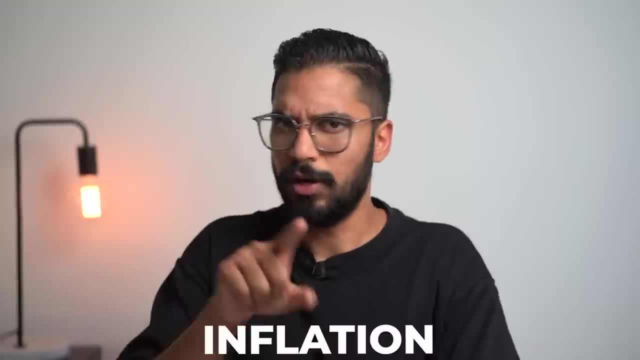 40 percent And then we're actually going to tax you again. It's called inflation, but you don't know it's a tax And effectively it's going to devalue the currency that you're holding, which means all the money you save you're just going to lose about three to five percent. 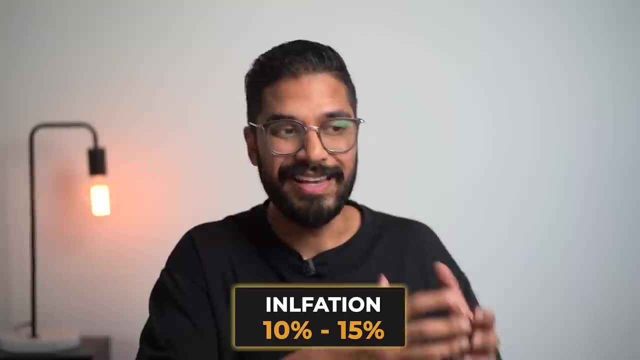 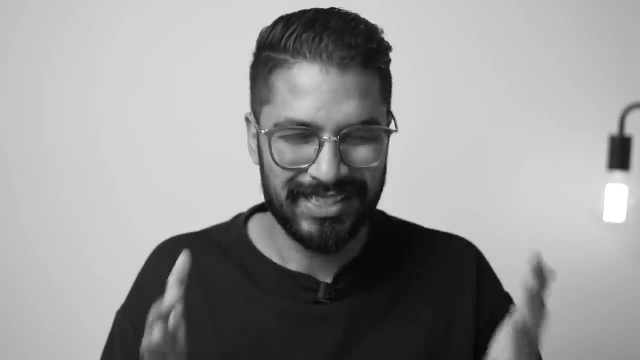 If you looked at true inflation, it's probably closer to 10 to 15 percent, And that's how much wealth is being lost, which is why, when you're saving your money, you often think about: hey, like I'm doing all the right things. People taught me to save my money, get into no debt. 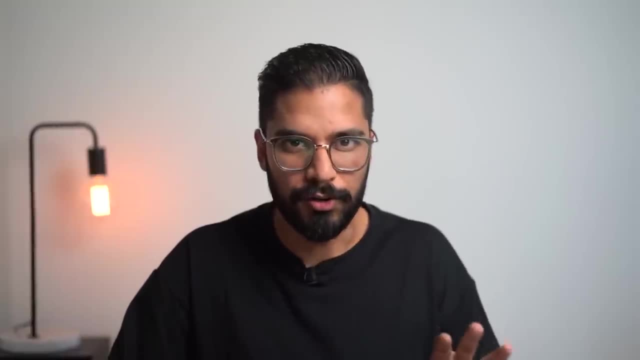 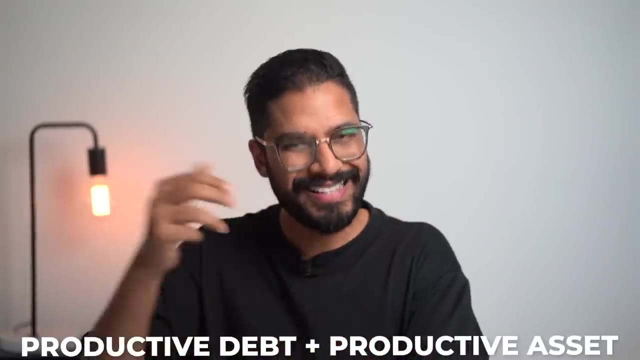 yet I feel like I'm falling behind. If you're someone that feels like you're falling behind, you're not alone. Smash that like button, because you'll know how many others are feeling the same way, And that's why we need to attach our productive debt to productive assets. That's. 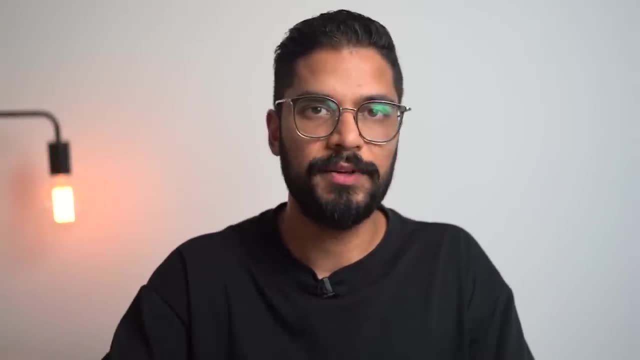 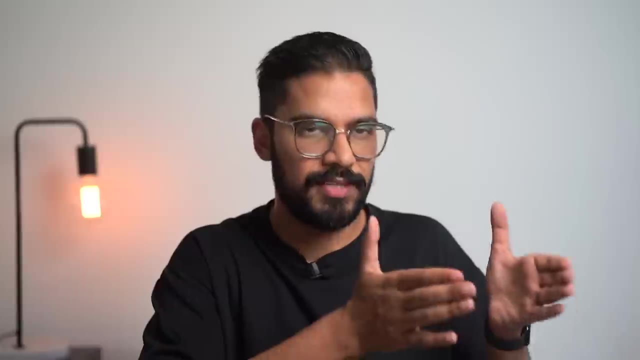 how you get wealthy. I believe we start seeing those interest rates cut in 2023, and that's going to start getting more people back into the market And they're going to say, well, if interest rates are cutting again, that means something's wrong with the economy, And if 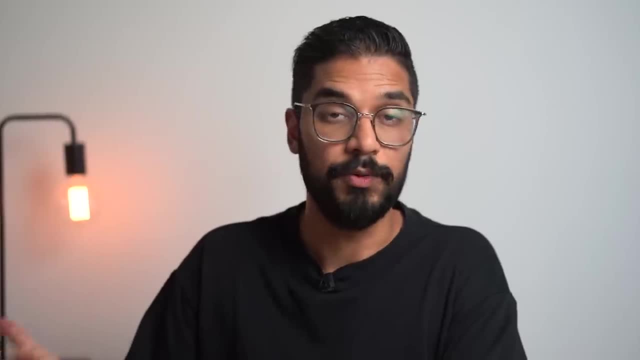 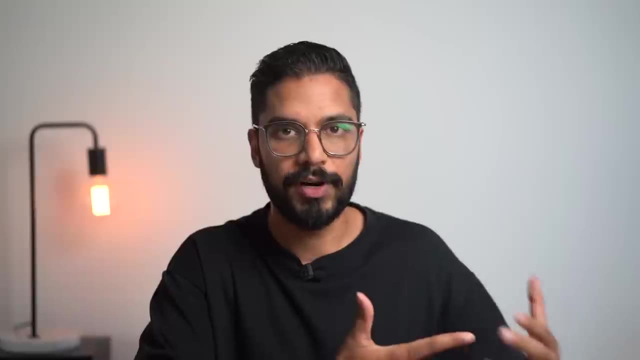 something's wrong with the economy. they're going to continue printing money or increasing liquidity. that means property prices go up. Let's get involved As a side note. that might potentially decrease the pressure we have on the rental market, because more renters will now be able. 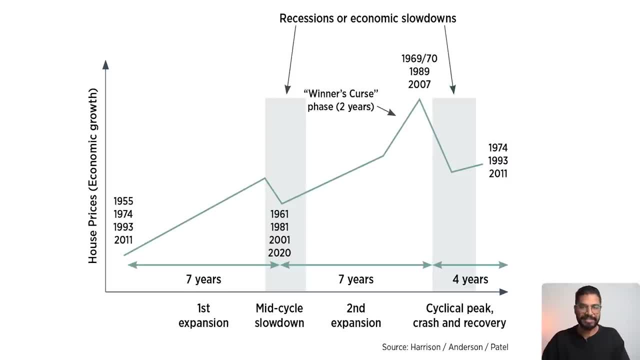 to afford to buy a house. Now the final graph I actually have is the 18.6 year cycle developed by Phil Anderson. Now there's a lot going on here. I'm going to break it down as quickly as possible for you. But essentially, what Phil Anderson believes in is this cycle that we have basically. 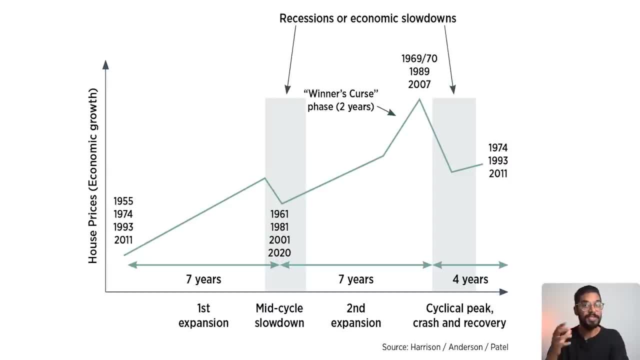 the first expansion, followed by the second expansion, But in between we have a mid-cycle slowdown And then we have some sort of blow off top before we have some sort of big correction in the market. Now, if you look at this- and we're going to use the most recent dates- if you look 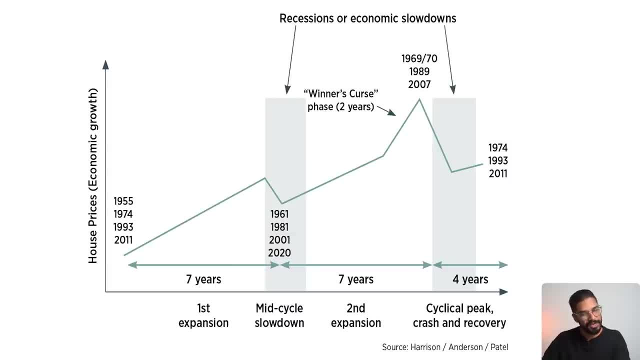 at 2011,. the first expansion part started. you go for pretty much seven to nine years, And then we ended up in 2020, where we did see a bit of a slowdown. Now, if you really think about this, in 2020, we actually had increases, So it wasn't really a slowdown, But what we actually saw was a year to two years prior to that, in 2018 and 2019, where the Australian market did slow down a lot. So when you're looking at this, don't think about: oh, that's the exact year I'm going to. 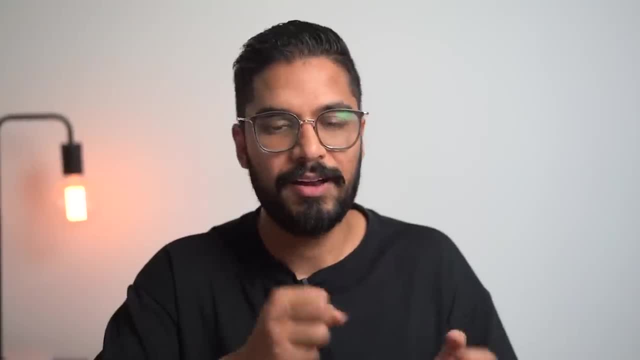 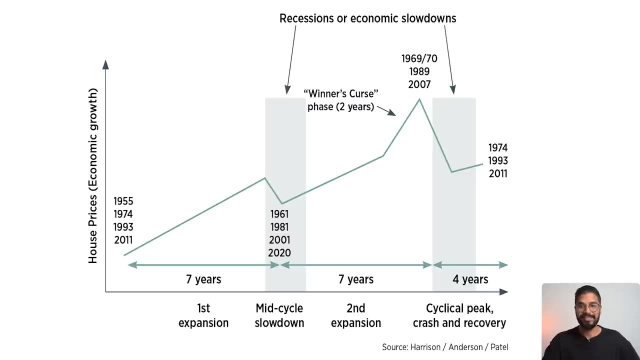 buy And that's the exact year that I'm going to sell. No, these cycles will play out, but they slightly different every time they do play out. So if we use this as an example, we could see that, based on this graph from 2020, another six years from there- we should see the top And that 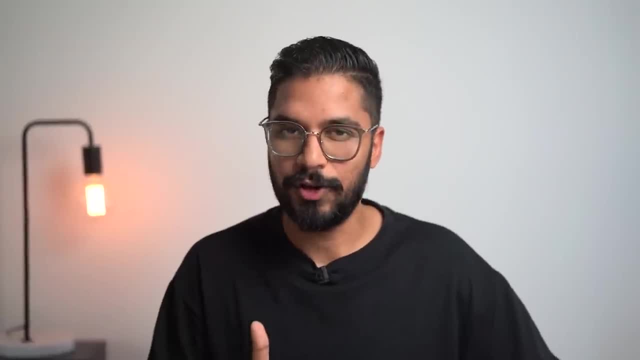 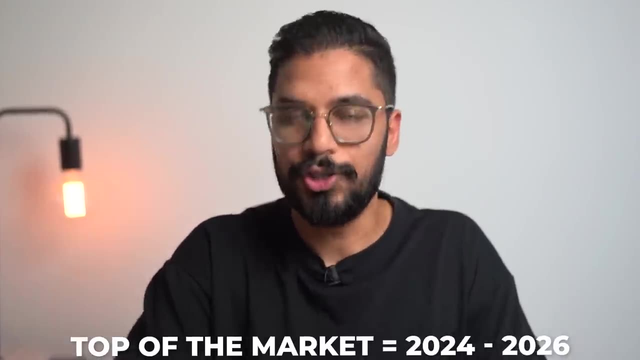 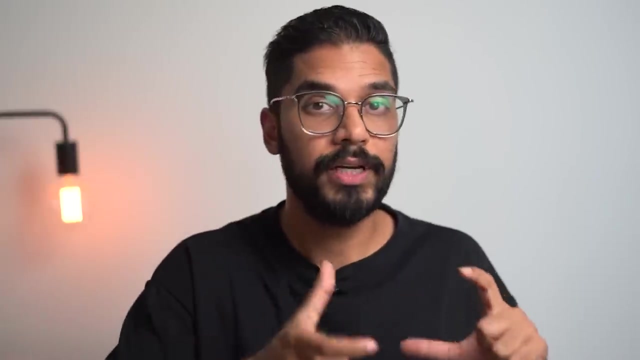 would effectively mean 2026. But if we started our mid-cycle slowdown in 2018 and 2019, that means the potential top for this market could look anywhere between 2024 to 2026.. I personally believe it's going to be closer to 2025 than it is to 2024.. And this would also tie in really well. 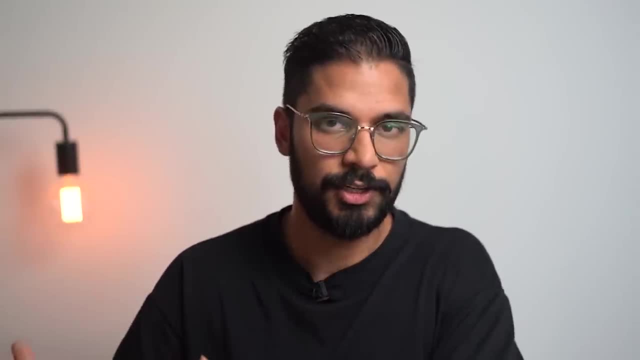 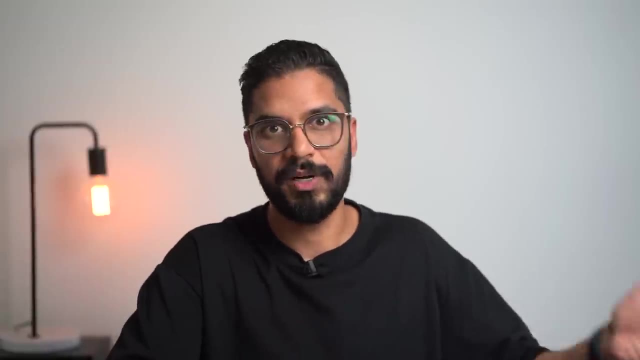 with how we're seeing the financial system change when it comes to blockchain technology And when you look at the next cycle for the Bitcoin halvening and how cryptocurrency has this massive blow off top that is positioned to be in 2025 as well. Could we see in 2025,? 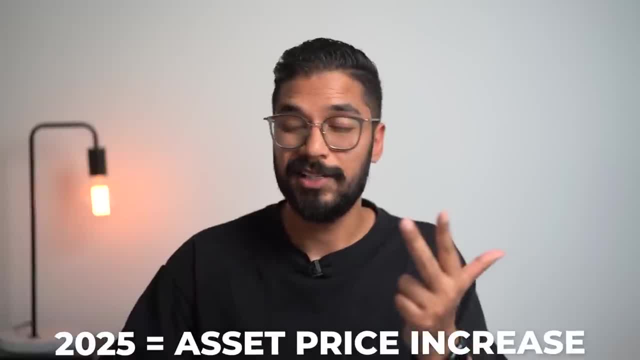 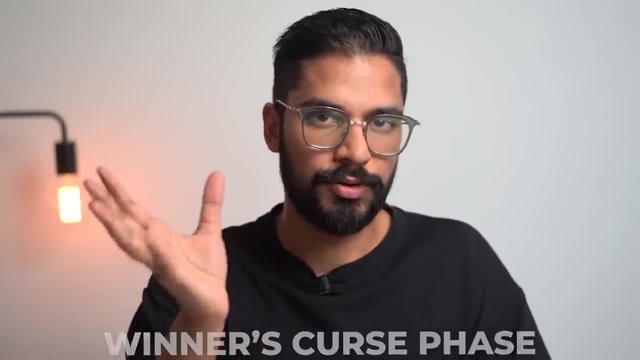 a mass devaluation of our currency, inflation going through the roof and asset prices absolutely taking off? Yeah, I think so. And that last phase, which is often referred to as the winner's curse phase, is where you get exponential growth Right towards the end, where there's FOMO buying And 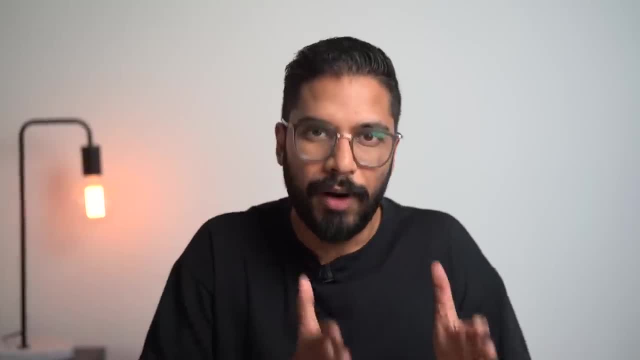 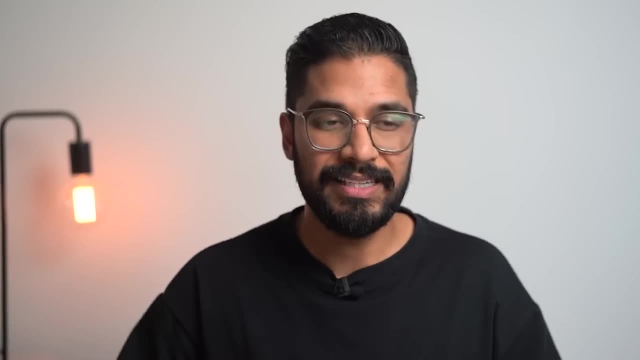 that's. what I mean is, if you're going out there in a market like now, you want to go and buy at time. You don't want to go and buy when everyone says the prices are going to go up and they're going to go up by 20, 30%. It's amazing. There are articles out there at the start of 2022 that 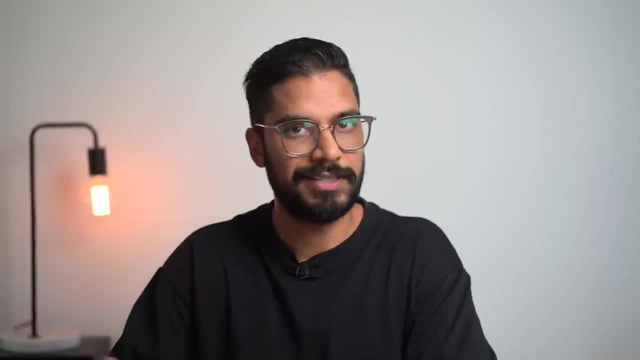 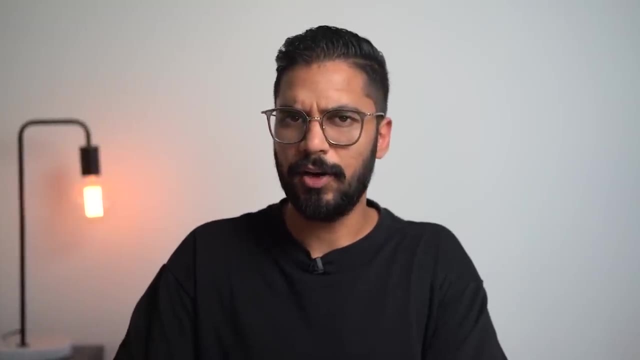 were saying, yes, property prices are going to go crazy this year, And that was before interest rates started increasing. But again, we knew the top was already in before that And the key follow-up question to something like this is: well, if I know that it's going to go up and 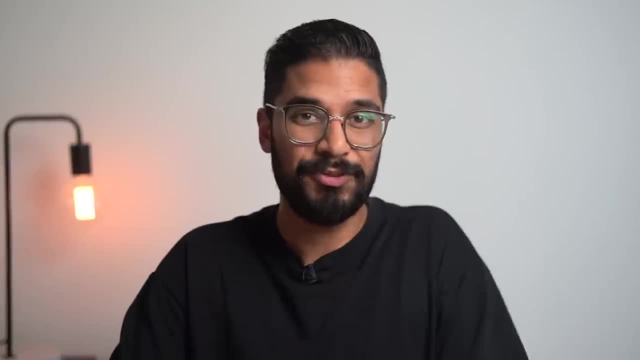 then it's going to correct by maybe 20 or 30%. should I sell at that point? Well, you're going to have to adapt And that's why you need the right team with you, Because if you don't have all the information, imagine you're like: oh yeah, cool, You know, I'm just going to do life now. 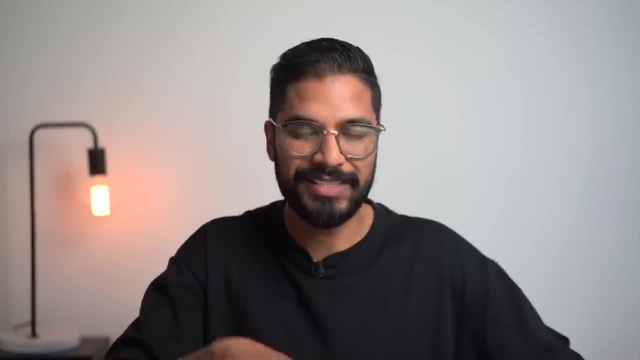 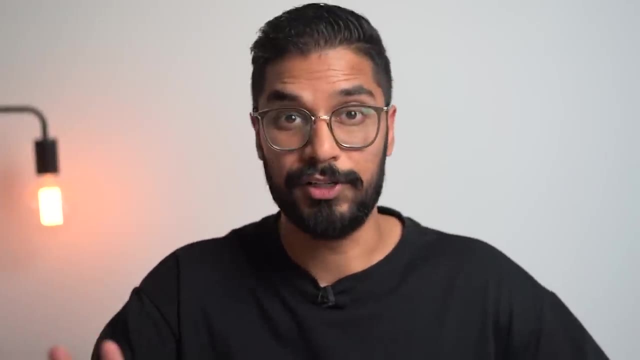 I've got a property portfolio. I've bought a couple of properties. You don't have a team that's actively in the market looking at what's happening. You're going to be six months too late, And six months too late when it comes to real estate is a hell of a lot of time That could. be the difference of maybe 10% May not sound like a lot, but if you've got a million dollar property and now it's dropped by 10%, you lose $100,000 and the anxiety and stress of the market going even lower. So timing is very important- If you can go and get time in the market as well as 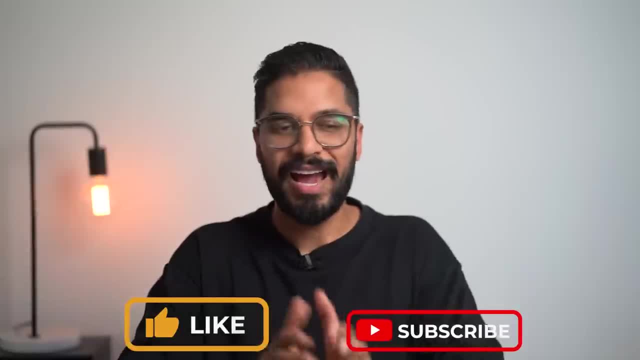 timing the market. you're going to do really well. I hope you guys have enjoyed this video. If you have, smash that like button, Subscribe if you haven't already, and check out all the other videos I've got on this channel. I'll catch you guys in the next one. Thanks, guys. 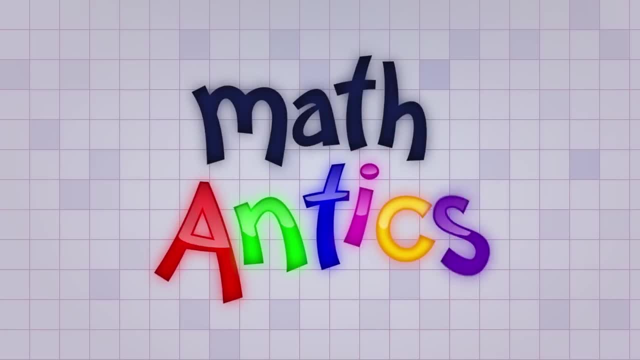 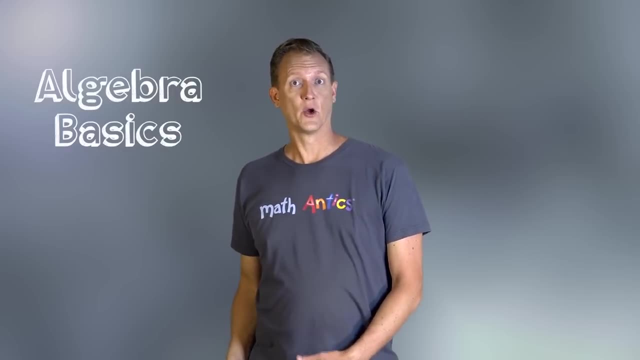 Hi, I'm Rob. Welcome to Math Antics. In this Algebra Basics lesson we're going to learn about functions. Outside of the realm of math, the word function simply refers to what something does, But in math the word function has a more specific meaning.